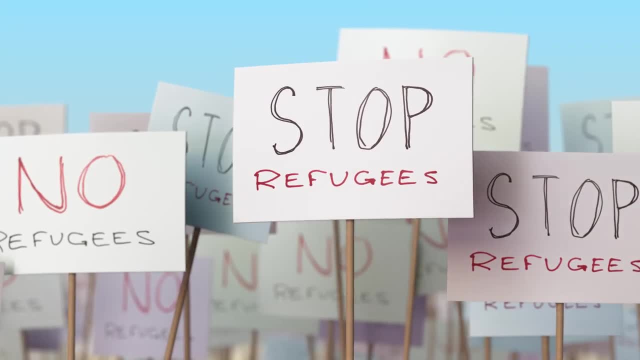 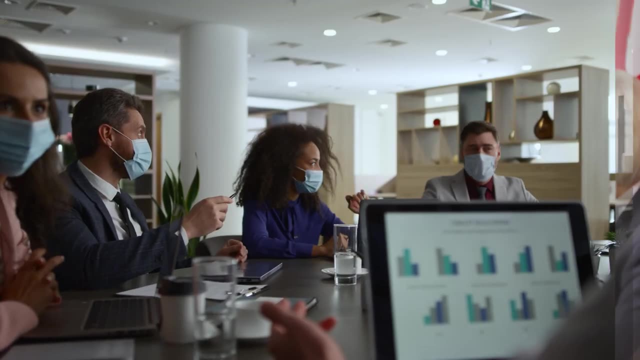 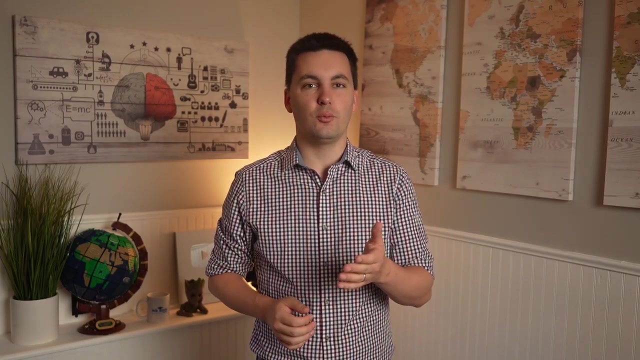 Certain governments may restrict certain migrant groups, such as refugees, while other countries may be more accepting. Traditionally, governments base their immigration policies around their economic needs, their national security priorities and also their country's cultural values. If a country grants an individual asylum, we can look to see how they help the migrant succeed in their new country. 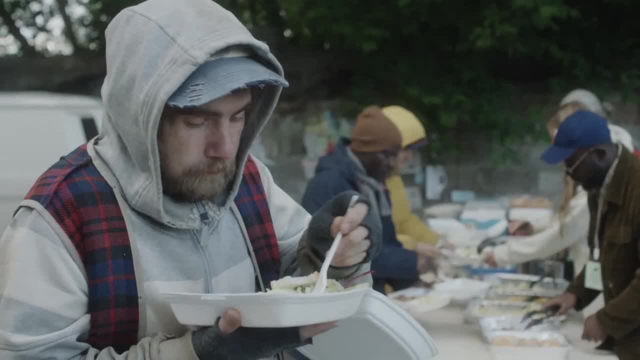 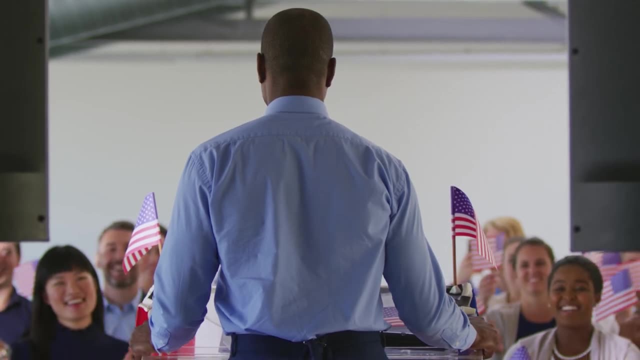 What systems does the country have in place to help transition the migrant, And how do citizens of the country treat the new migrant? Often times, a country's immigration and immigration system is different. Immigration and migration policies become heated debates in a country. Many countries today have debates over the amount of immigrants they should allow into the country. 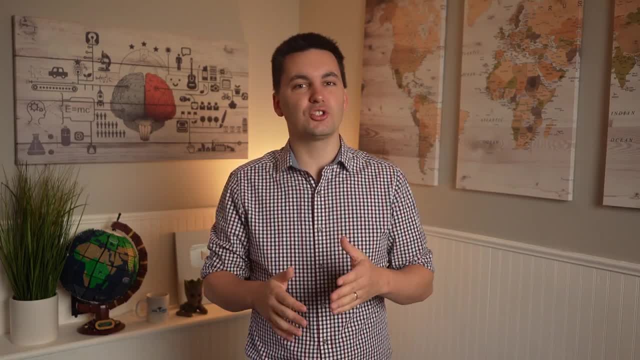 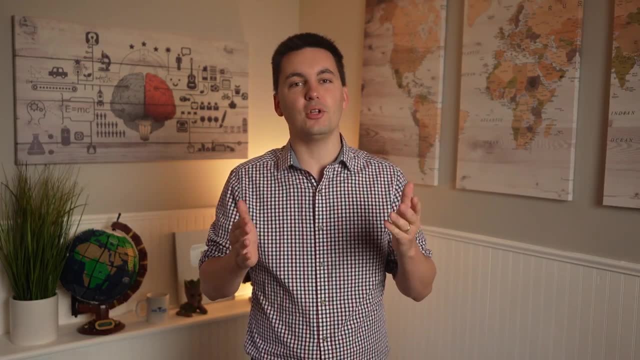 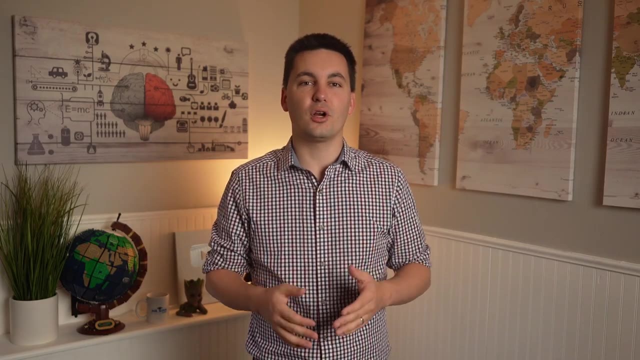 How the country should handle unauthorized migrants, How to enforce the country's borders, What services the country should provide migrants and immigrant groups, And what immigrants should be allowed into the country in the first place. Individuals who want to reduce the number of immigrants coming into a country will often be in favor of immigration quotas. 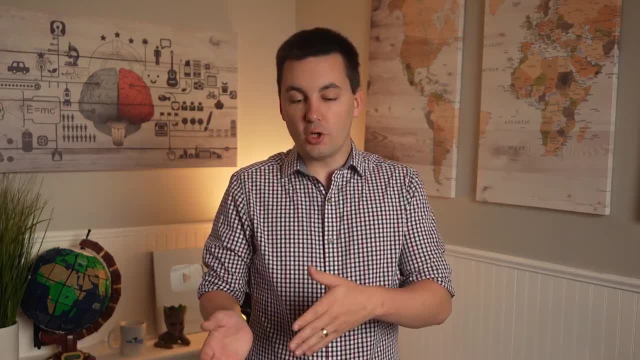 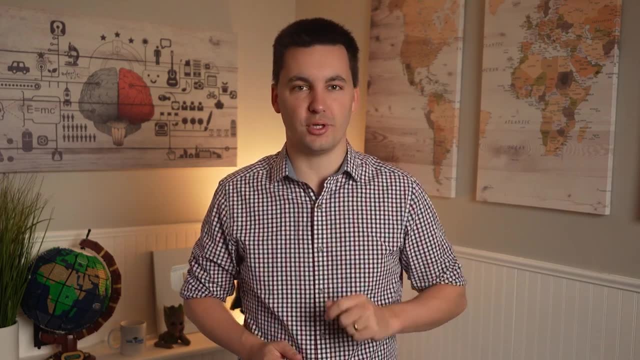 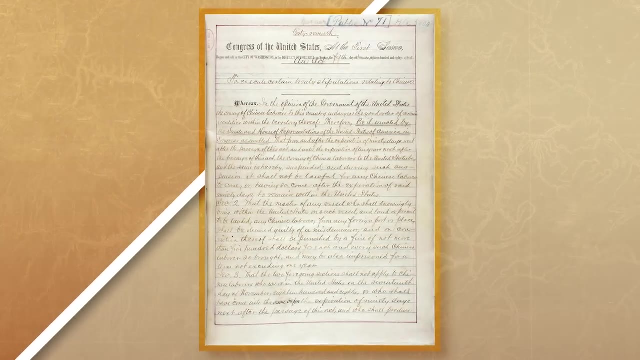 Which limit the amount of immigrants coming into the country. If we look back in history, we can see how immigration policies change over time and how they shape the demographics of a country. For example, in 1882, the United States had an anti-immigrant sentiment and passed the Chinese Exclusion Act, which restricted immigration to the United States. 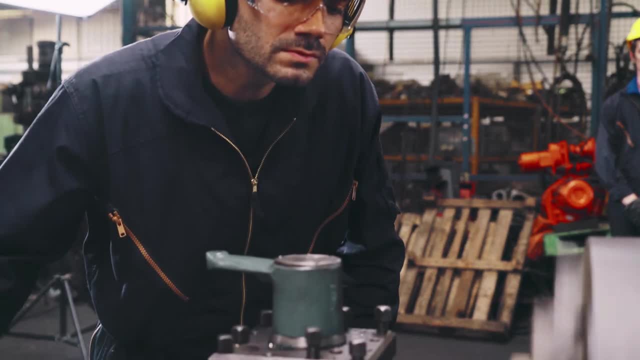 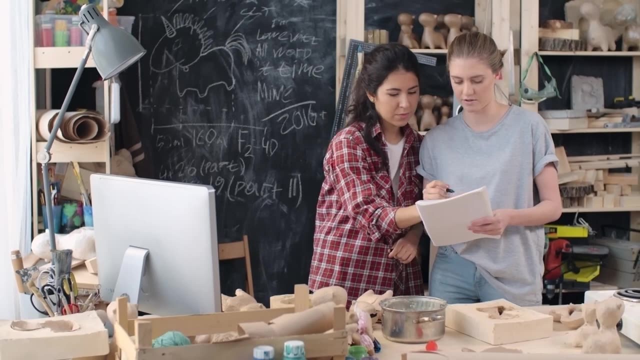 Economically, we can see that countries that have more immigrants often see an increase in their economic output. New immigrants create new businesses, help fill gaps in the workforce and bring new ideas into society. Now, countries that do not have as much to offer their citizens might experience brain drain. Which is when the skilled labor leaves the geographic area in favor of another area that offers more opportunities. This can put a strain on the economy, as society may no longer have the talent that it needs to expand the economy. When countries see more migrants entering the country, they gain access to a larger and more diverse workforce. 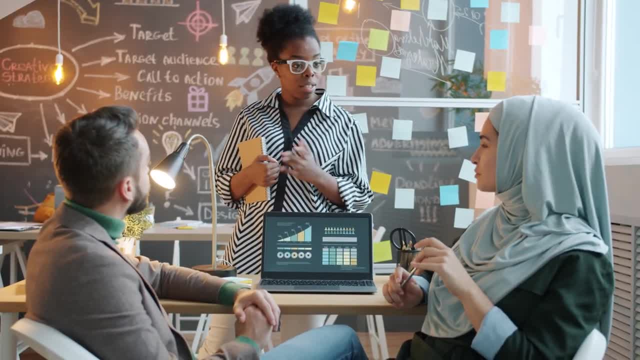 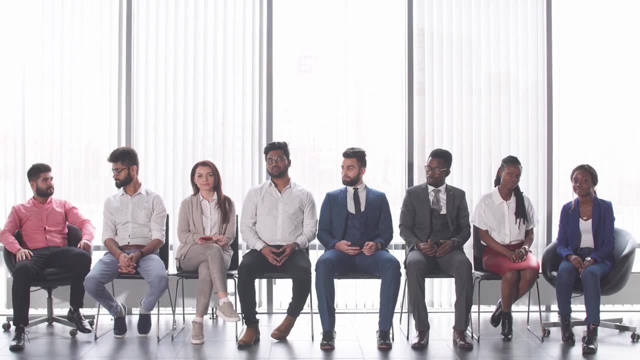 Which can lead to new innovations and more production, But, at the same time, will also make the job market more competitive, Which may reduce the bargaining power of the worker, Making it more difficult for individuals to get a job. We may also see immigrants take jobs away from individuals who have been previously living in the country. 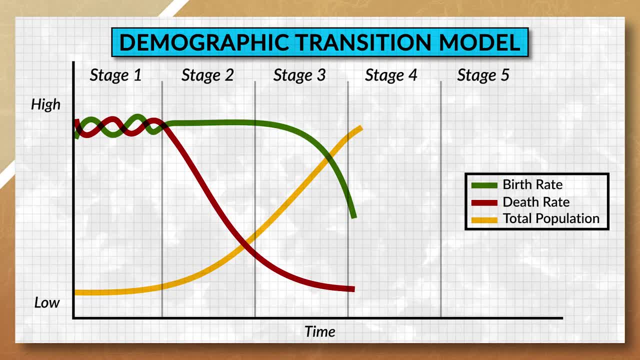 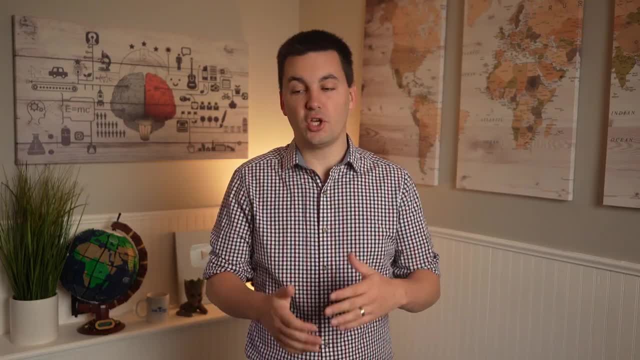 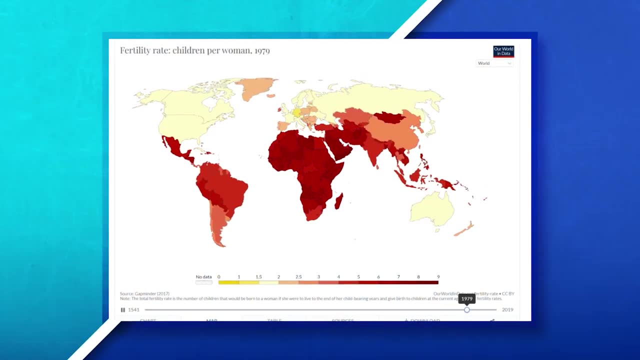 But if we connect back to the demographic transition model, we can see that countries that are in stage 4 of the model may end up relying on immigration to help stabilize their shrinking growth rate. If a country restricts immigrants from coming in and does not see their TFR remain above the replacement rate, they may have a shortage of workers.